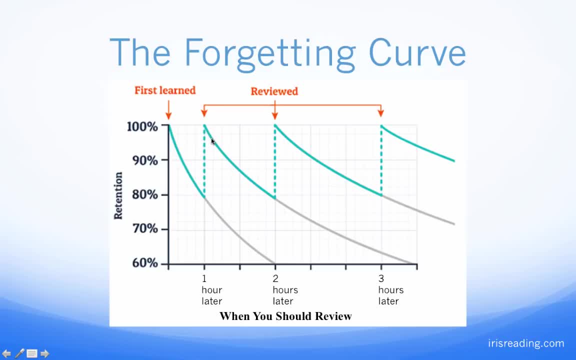 That's a very, very steep slope. Now, eventually, we review the information and then we start forgetting again, but it's not nearly as steep as it was earlier. Why? Because we reviewed it a second time. Now, if you review it a third time, 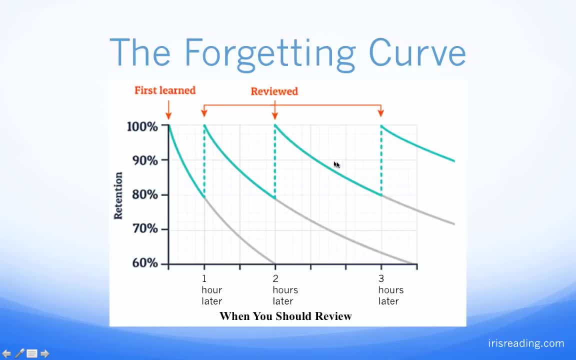 it doesn't get as steep. Notice how it's kind of leveling out more and more. The more you review something, the less likely you are to forget something. Now we all know that. but the question comes down to when exactly should I review? So this might be, let's say, an hour. 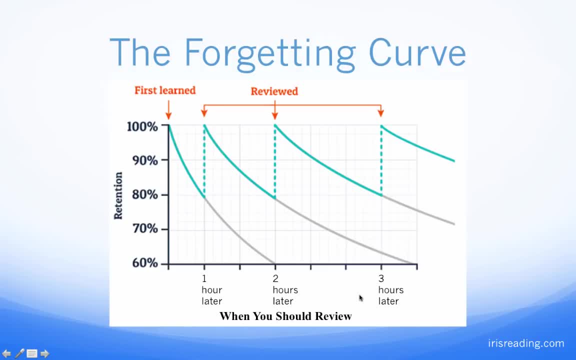 later, two hours later, three hours later. It comes down to what's the optimal amount of time, and when should I review something? Well, it turns out we already know that the more we review something, we're going to forget something. So we're going to forget something. So we're going to. 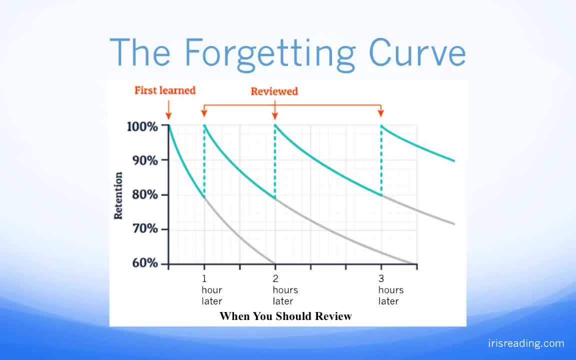 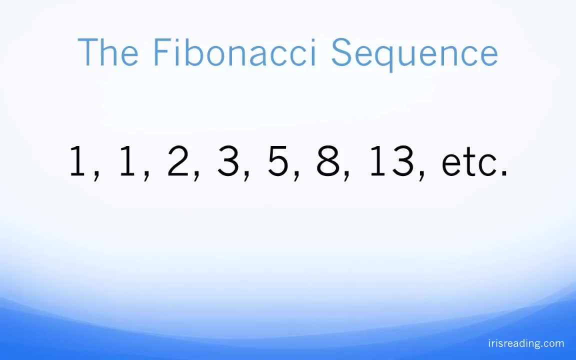 the less often we have to review it, because every time I review it I retain it a little better. So you can utilize something called the Fibonacci sequence in your study plan, And some of you are probably familiar with the Fibonacci sequence. Basically it's a sequence of numbers where you 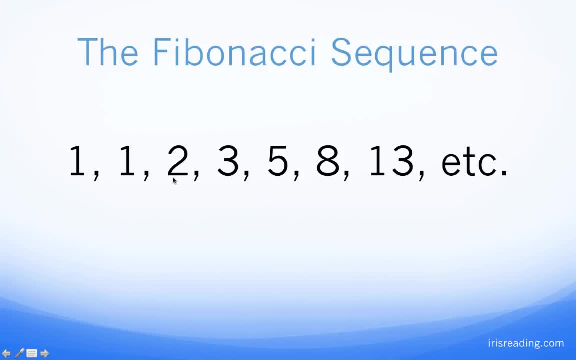 have the first two numbers and they will give you the next one. So one and one gives you the sum of one, and one is two. One plus two equals three. Two plus three equals five. Three plus five equals eight, and so on and so forth. That's a Fibonacci sequence, So you can utilize something called the. 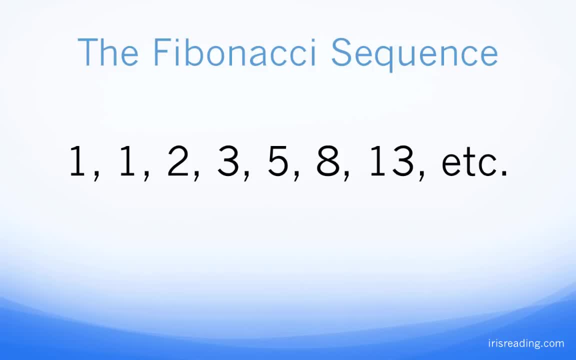 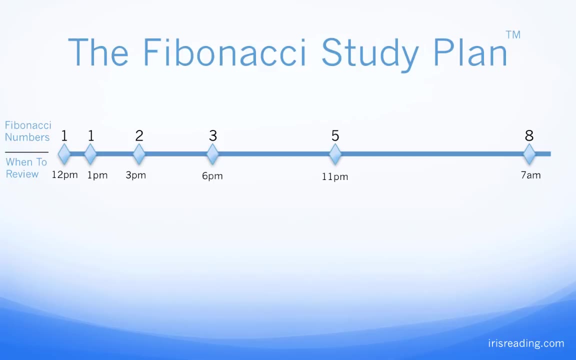 Fibonacci sequence. And the Fibonacci sequence has all sorts of applications, from nature to many other things. I'm not going to go into detail on those. I want to talk about how you can utilize it for studying, And this is where the Fibonacci study plan comes into relevance. So at the top, 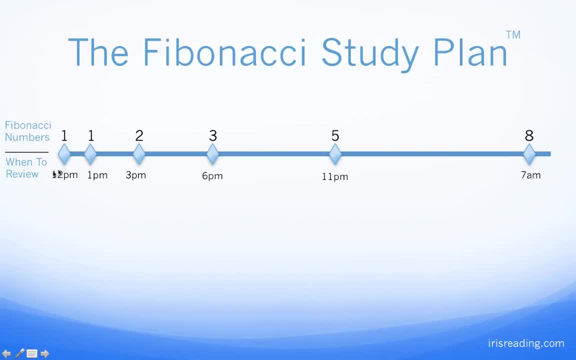 here we have Fibonacci numbers. At the bottom we have a schedule of when to review. So this is just an assumption of, let's say, we start our review at 12 pm, And when I say review, this might be reviewing your notes, reviewing vocabulary or anything else that you really need to learn Maybe. 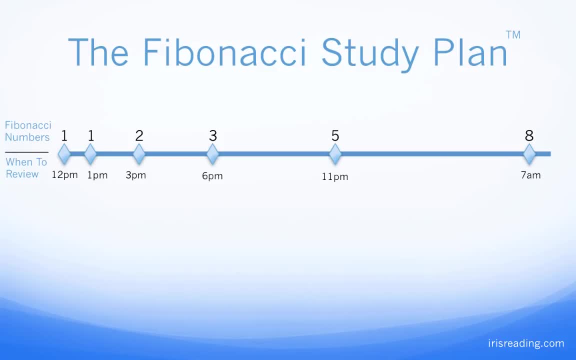 you've got a test coming up. Maybe you have a presentation coming up at work. So let's say we review the information at 12 pm. Now our next Fibonacci number is one, So one hour later is when we would review at 1 pm. The next Fibonacci number is two, So two hours later that's 3 pm. 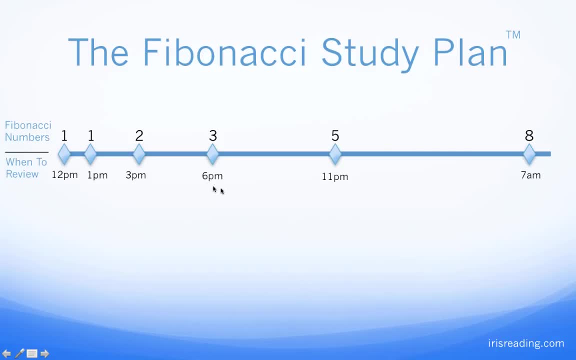 Now, three hours later, that's 6 pm, Five hours later is 11 pm, And then eight hours later is 7 am. Now this conveniently works out to overnight, So we get to sleep And there's a lot. 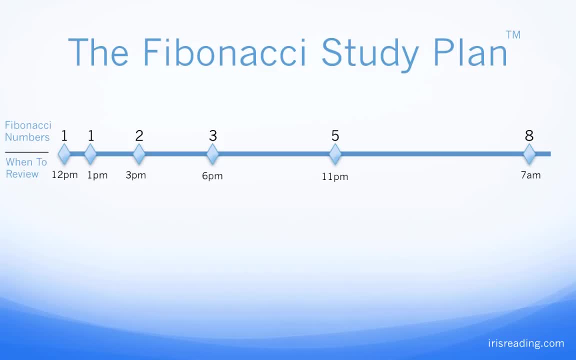 of benefits to learning something or reviewing something before you go to sleep. There's a lot of research on that- And then, of course, first thing in the morning. Now, at this point, whether or not you want to continue going on, you could quit at any of these points. How far do you take this? 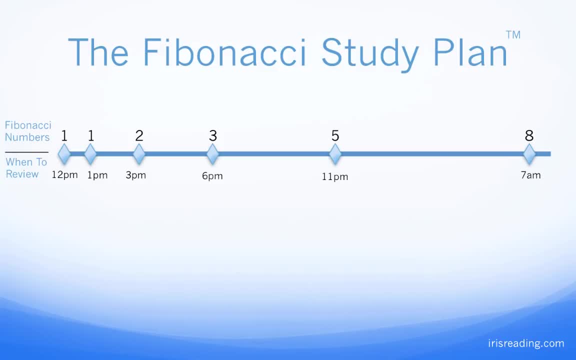 depends on how well you need to know it. You do more repetitions for information. you need to know very well, And this also depends on you know. at this point, after you've had this many repetitions, let's count them: one, two, three, four, five, six repetitions. at this point you might feel 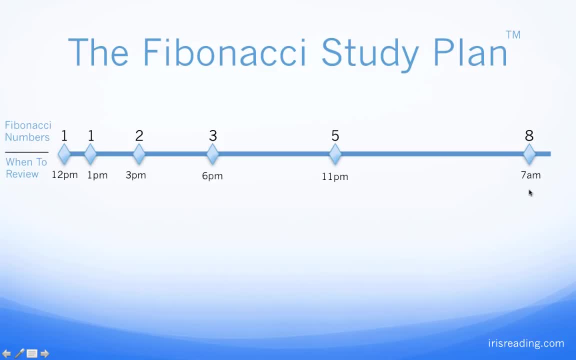 very confident that you know this information inside out Now. if you don't, you'd want to review the information again. But our next Fibonacci number would be 13.. Five plus eight equals 13.. Thirteen hours later, that would be 8 pm the next day. So well, 8 pm of the same. 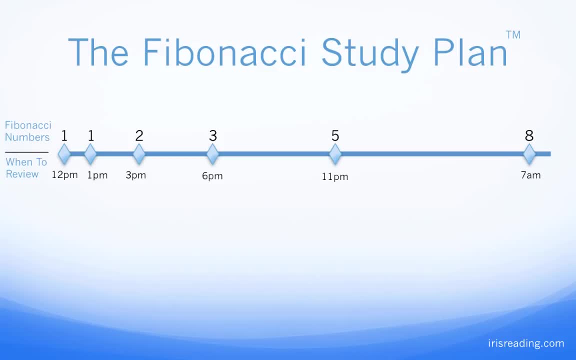 day, if we're comparing to 7 am. So the Fibonacci study plan allows you to have some structure with regard to your study. If you do all these repetitions in the span of 15 minutes, it's not going to be as effective as spreading them out, And spreading them out while taking into account. 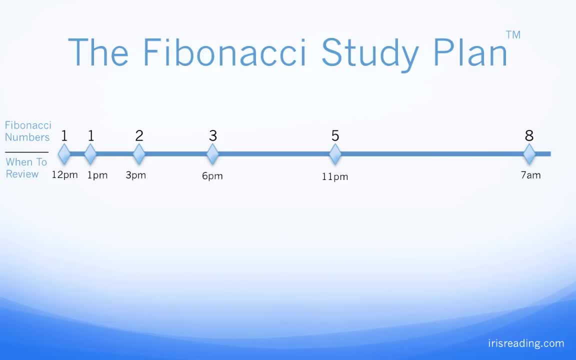 the Fibonacci sequence is an optimal way of studying Now. I mentioned at the beginning of this video that if you stuck around to the end, I'd give you a little secret. This is actually experimental with regard to our YouTube audience. What I did just a few minutes ago is I set up a 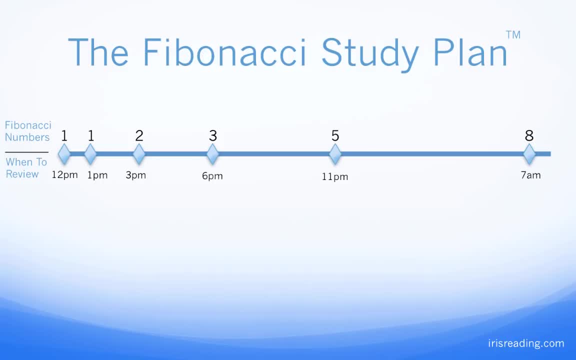 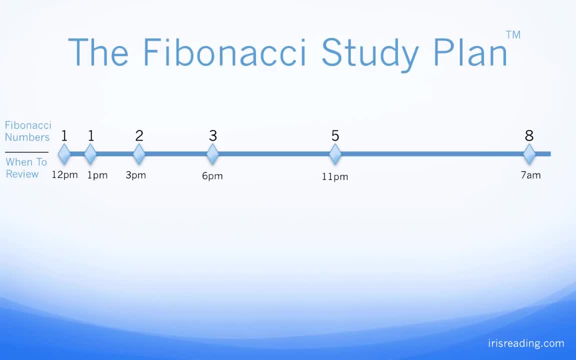 offer. It's going to give you half off of anything, And that's on top of any discounts that we already have on the website. So 50% off if you enter the code TUBE- Not YouTube, but just TUBE T-U-B-E.